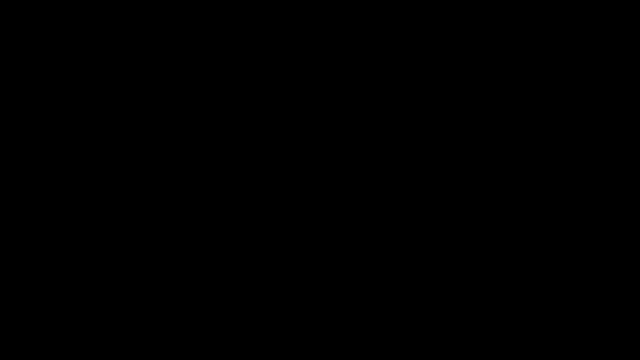 In this video, we're going to focus on naming organic compounds, particularly alkanes. So let's start with a simple example. How can we name this alkane? Well, we need to identify the number of carbons in the parent chain, And so 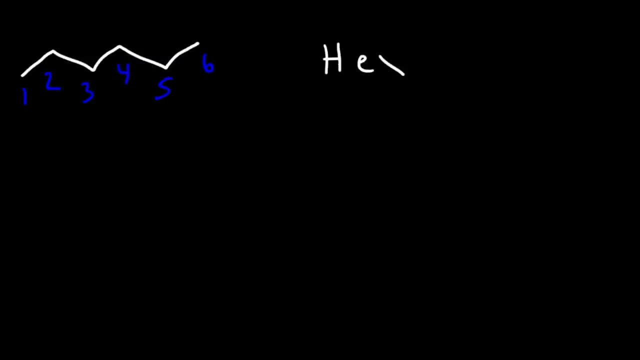 because it has six carbons. this is called hexane. Now, keep in mind: one carbon is methane, two carbons is ethane, three is for propane, four is for butane. five carbons is pentane, seven is heptane, eight is octane, nine is nonane. 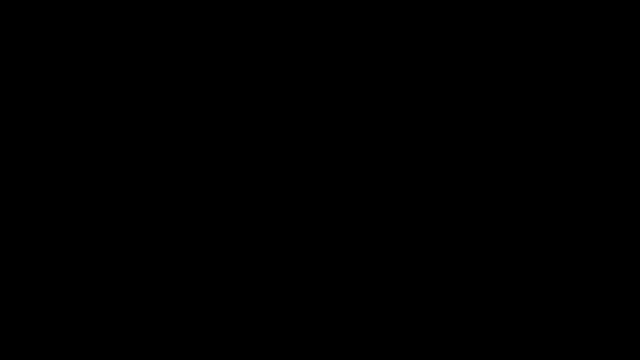 ten is decane. Now, what about this example? How can we name this particular alkane? The first thing you want to do is count the number of carbon atoms in the parent chain or the longest chain. Now, should we count it in this direction or 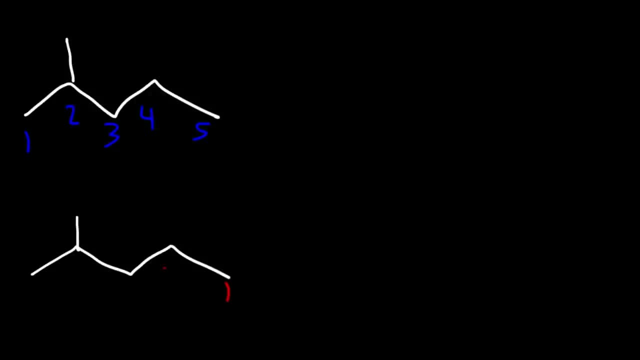 should we count it in this direction? The methyl group that we see here is called a substituent, and you want to count in such a way that the substituents have a lower number and 2 is lower than 4.. So this is the correct way to count it. So 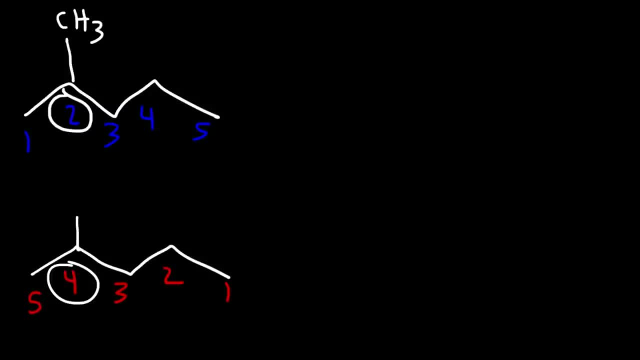 how can we name it? We have a methyl group on carbon 2, and there's five carbons in the parent chain, so this is going to be called 2-methylpentane. You need to use a hyphen to separate a number from a word. 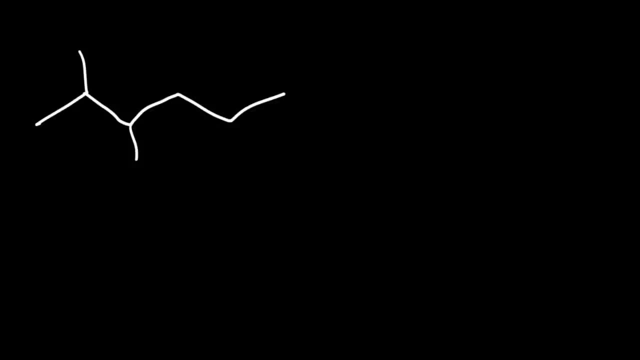 Now, what about this example? So clearly we need to number it from left to right rather than right to left, because we want the substituents to be 2, 3, instead of 4 and 5. if we counted it in this direction, So 2 and 3 are lower than 4 and 5, so we're going to use this. 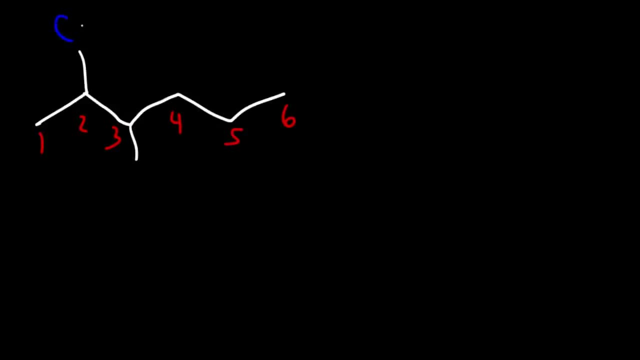 example, Now we have a methyl group on- okay, this computer is having issues now, so we have a methyl group on carbon 2, and on carbon 3.. So how can we name it? in this case? So the parent chain is hexane, because it has six carbons and there's two methyl. 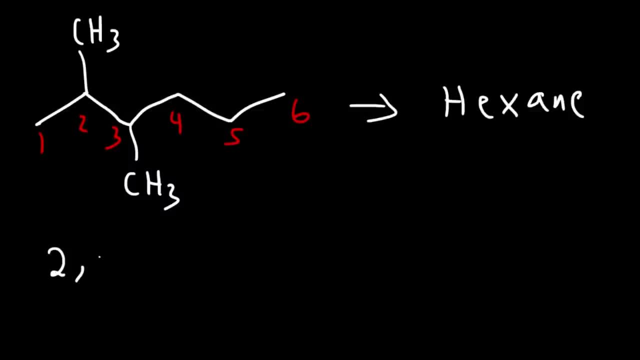 groups. so how can we write this? So you need to write 2, 3-dimethyl. di is for 2,, tri is for 3,, tetra is for 4, so it's dimethylhexane, If you have. 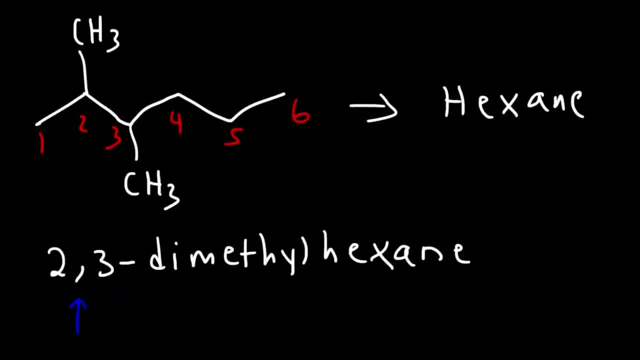 multiple substituents, then you need to use a comma to separate them. By the way, when you get a chance, check out the description section of this video. I'm going to post a few links, particularly my Patreon page, where you can access the organic chemistry 1 & 2 final exam preparation videos, if you're. 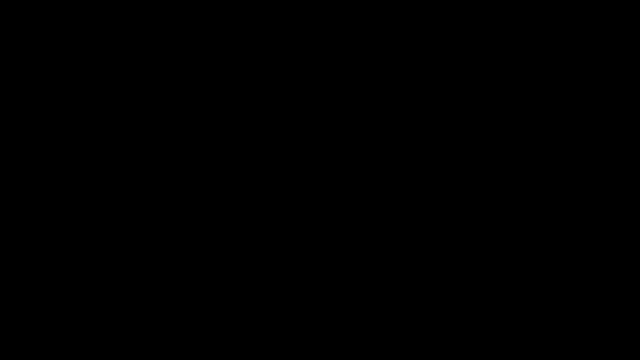 currently studying for that, So feel free to take a look at that when you get a chance. I'm going to post some other links to some other videos as well that you might find helpful too. Now, what about this example? Now, what about this example? 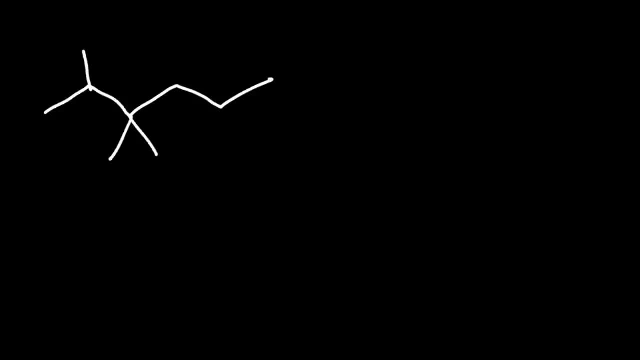 Go ahead and type your answer and type your answer into the chat. Go ahead and name that particular alkane. So we're going to number it from left to right, because it's going to give us the lower numbers And this time we have three methyl groups as opposed to two. 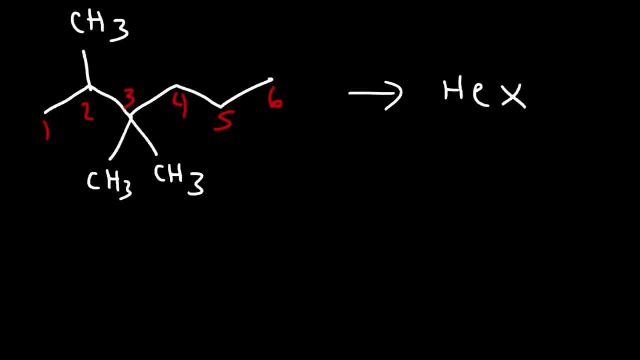 So the parent chain is still hexane, And so let's put it all together. So we have a methyl group on carbon 2, and we have two methyl groups on carbon 3. So we have to write 3, 3.. You don't want to write the 3 just once, You need to write it twice, because there's two of them on carbon 3.. And then we'll need a hyphen trimethyl, because there's three methyl groups. And then the parent name hexane. 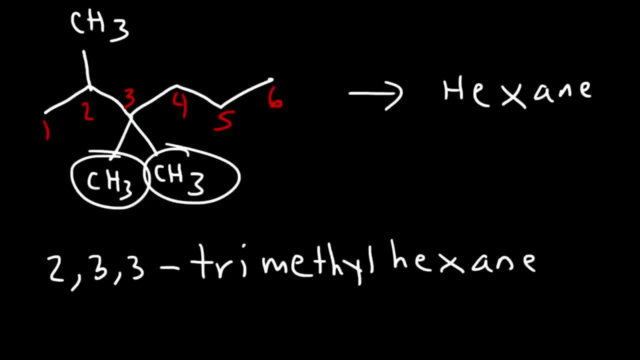 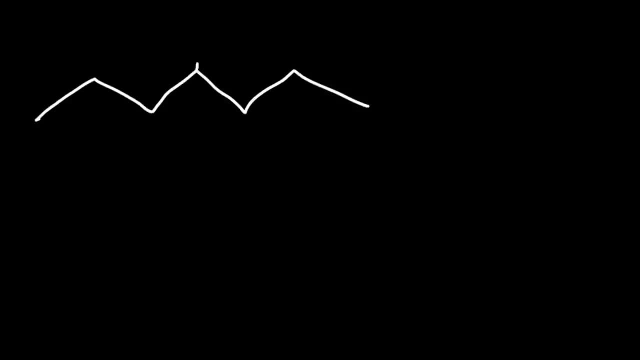 So that's how we can name this particular organic compound. Here's another example for you. Go ahead and try that problem. So we'll need to number it from left to right, And it looks like we have a methyl group on carbon 3.. 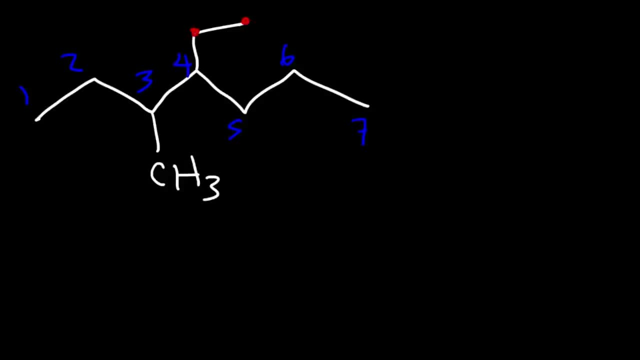 And on carbon 4, we have a substituent with two carbons, So that's an ethyl group. Now how should we name this? How can we put this together? Should we name it as 3-methyl-4-ethyl? 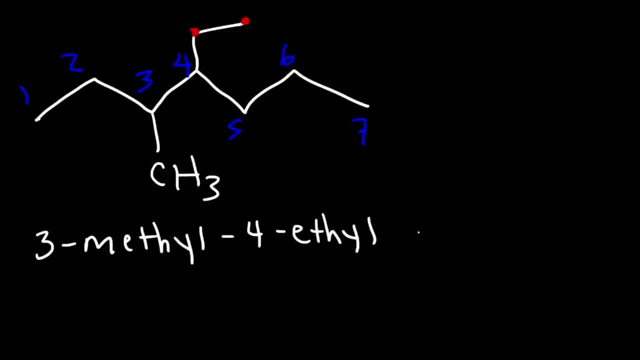 And the parent chain has 7-methyl-4-ethyl, So that's 7-carbons, so that's heptane. Or should we say 4-ethyl-3-methyl-heptane? So which of these two names is correct? 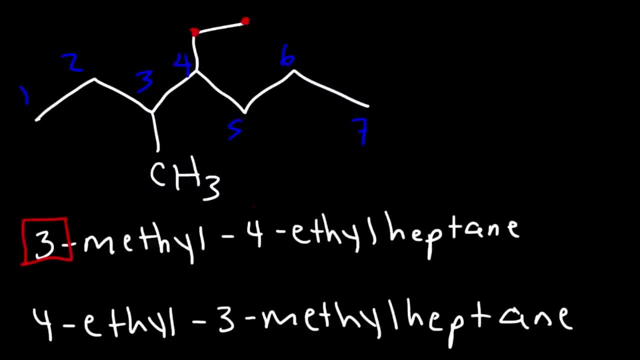 Now looking at the first example, the numbers are arranged in increasing order. Now looking at the second example, We could see that it's arranged in alphabetical order. E comes before M. So which one should we give more priority to: Arranging the numbers in ascendant order or putting the letters in alphabetical order? 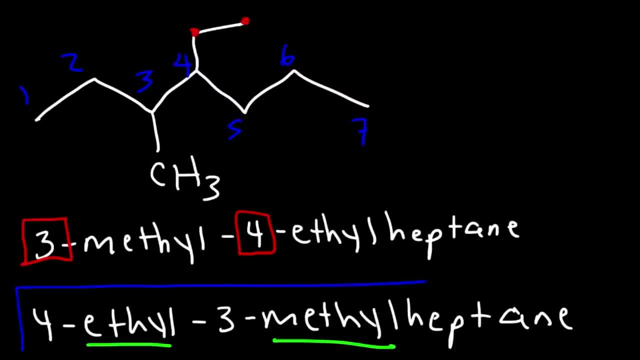 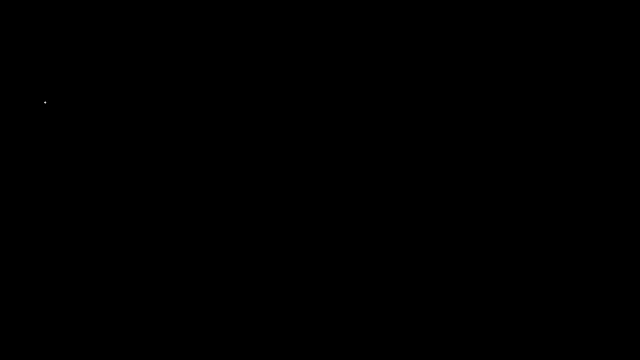 It turns out in this situation you need to alphabetize the substituents. So the ethyl group must come before the methyl group, regardless if the numbers are increasing or decreasing. So this is the right answer. Now let's move on to our next example. 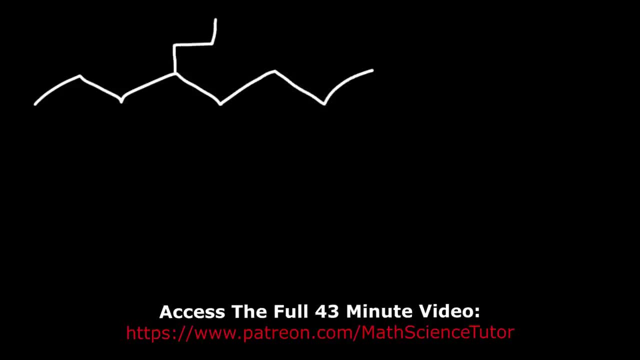 So notice that we have a propyl substituent- There's three carbons- And we have an ethyl substituent. How do you think we should name this particular molecule? If you want to pause the video and try the problem, feel free to do so. 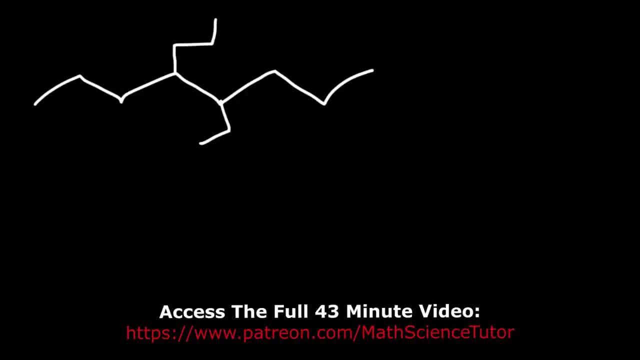 Now, what direction should we take? What direction should we count this molecule? So let's count it both ways. I'm going to redraw this structure. So in the first example, let's count it from left to right, And for the second example, let's count it the other way. 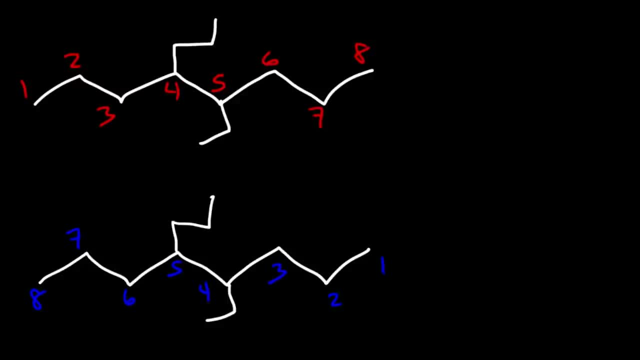 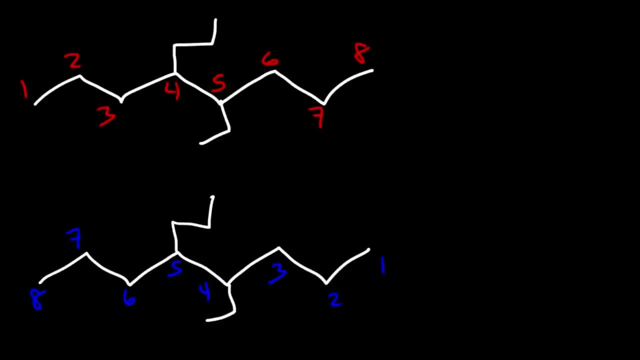 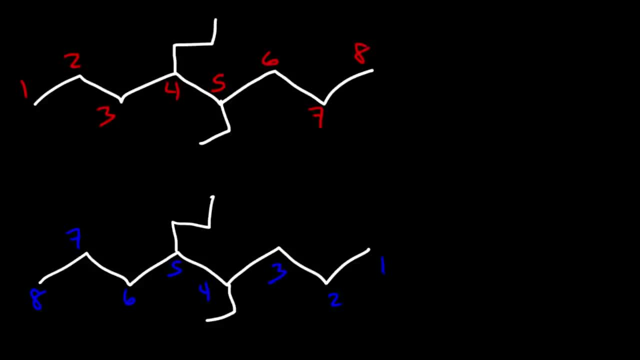 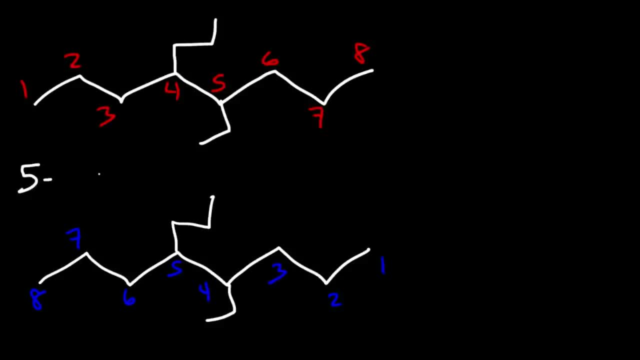 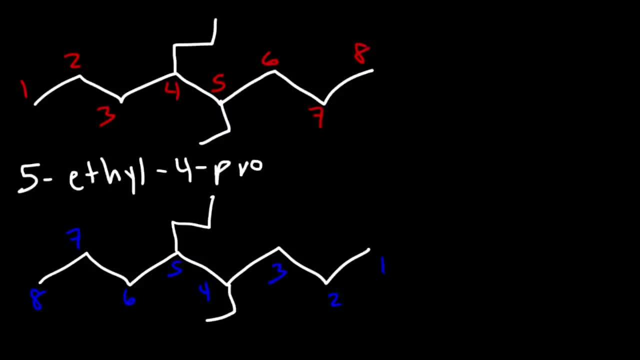 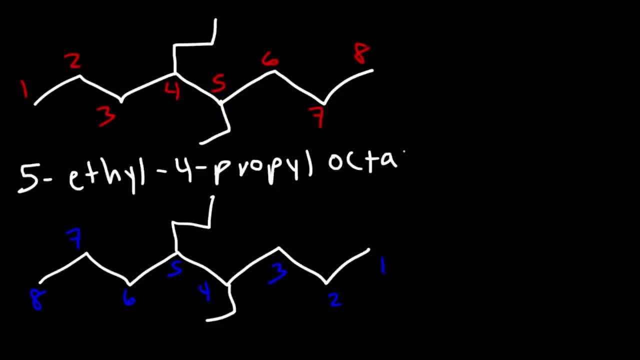 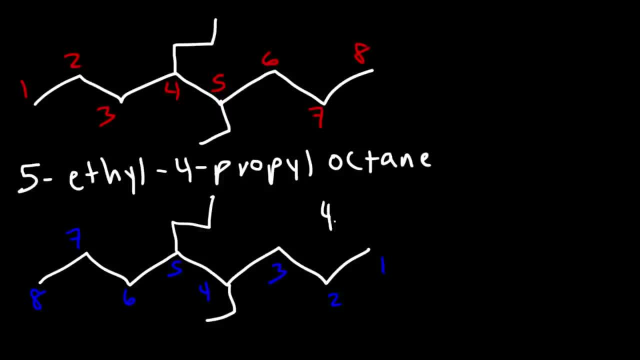 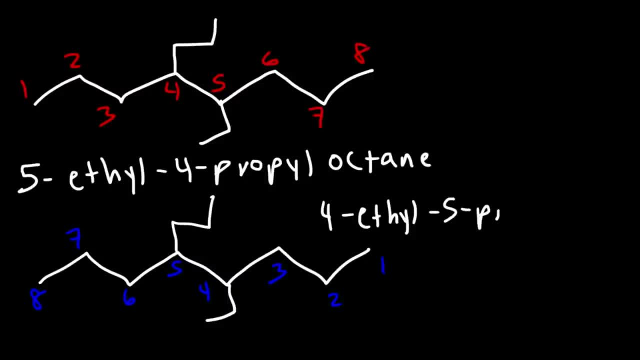 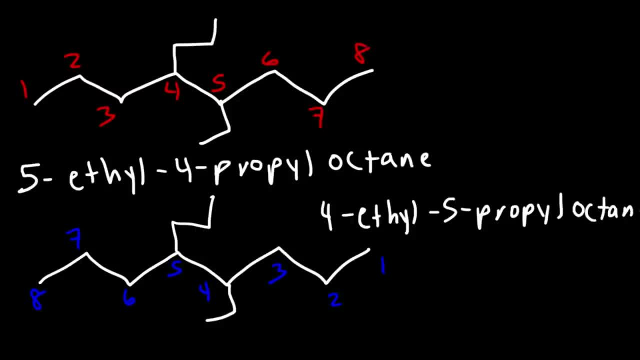 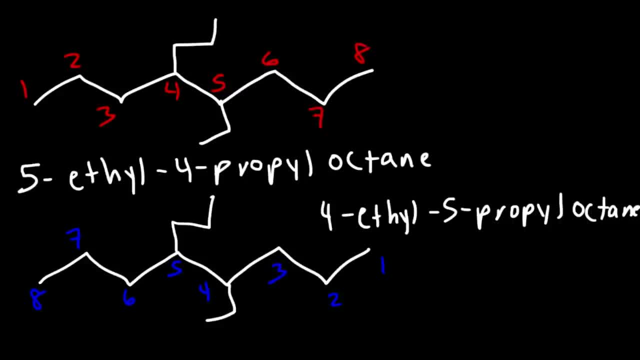 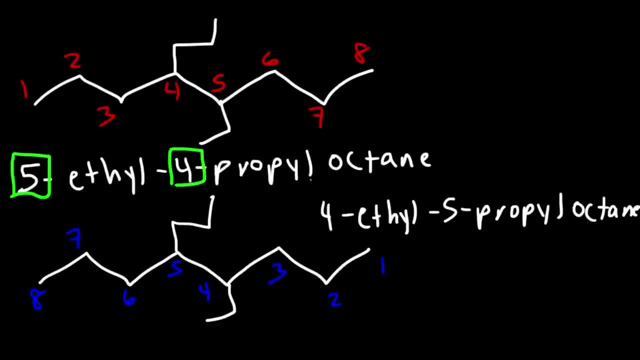 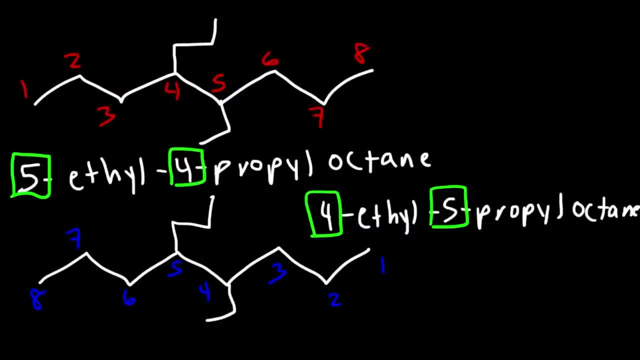 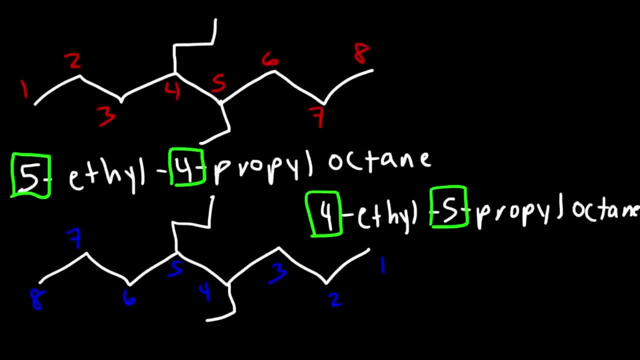 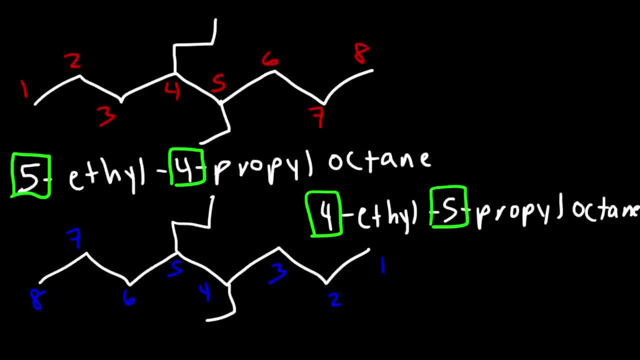 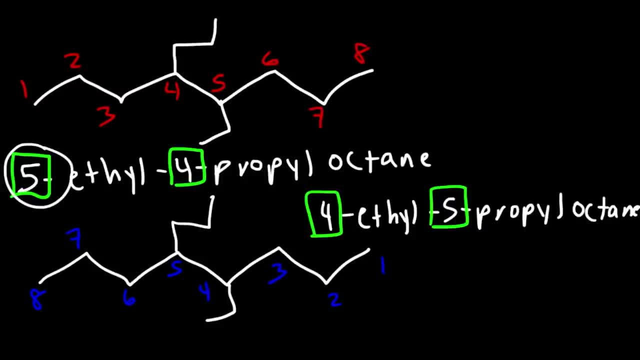 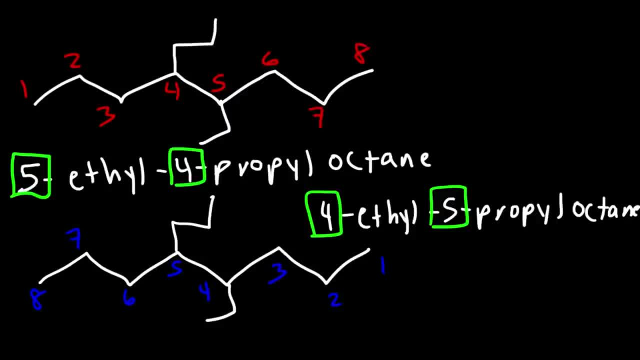 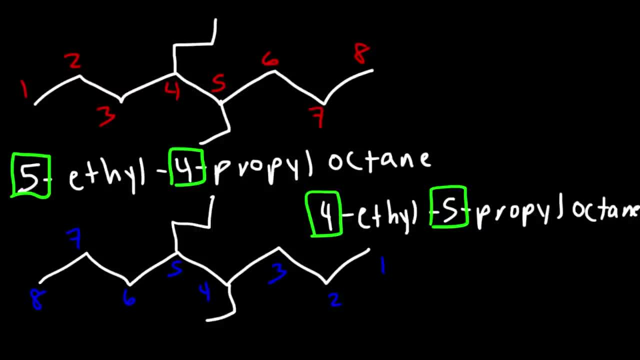 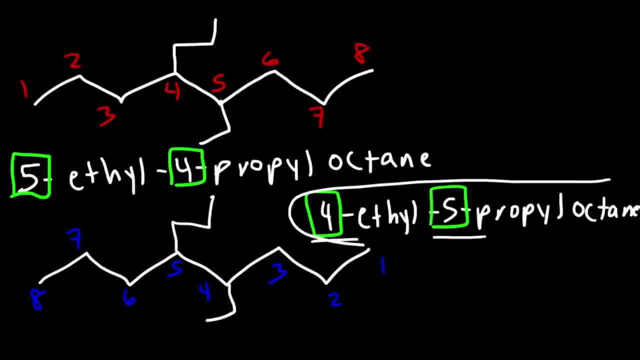 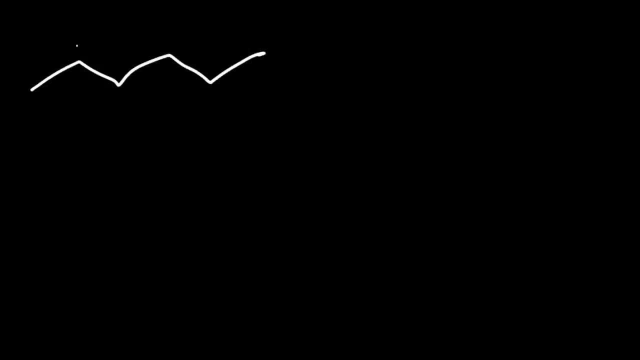 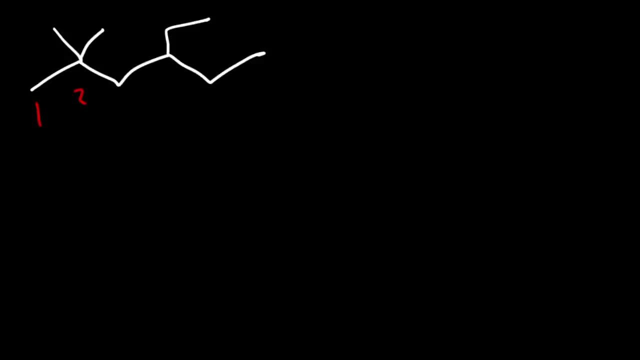 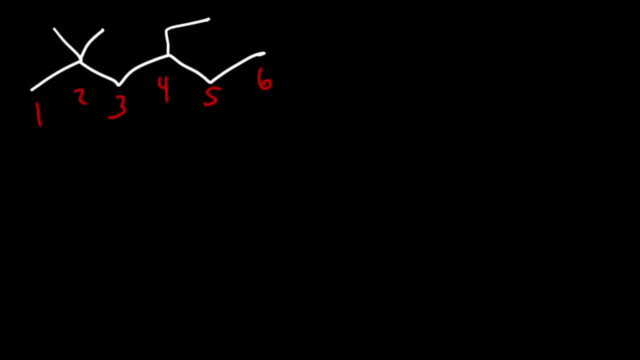 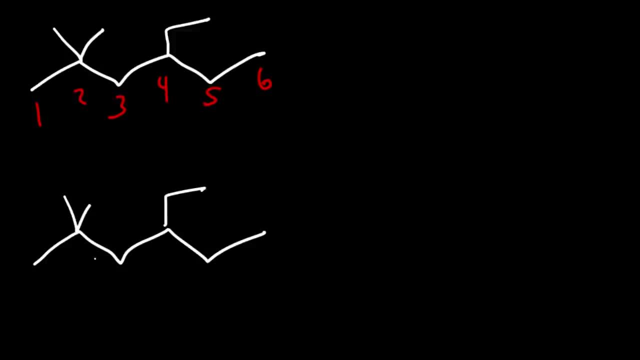 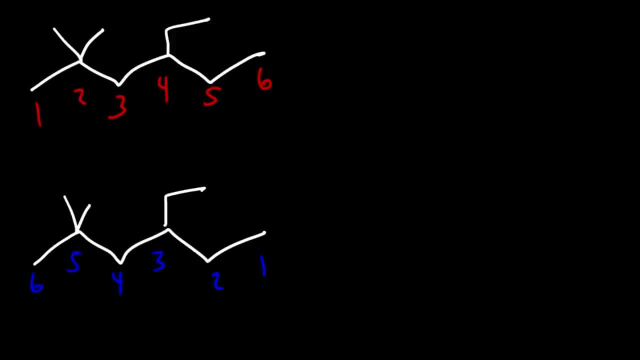 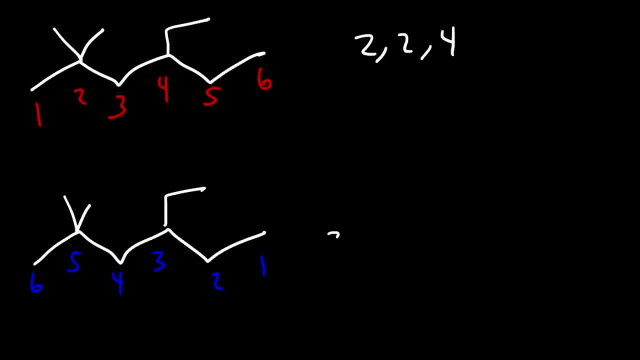 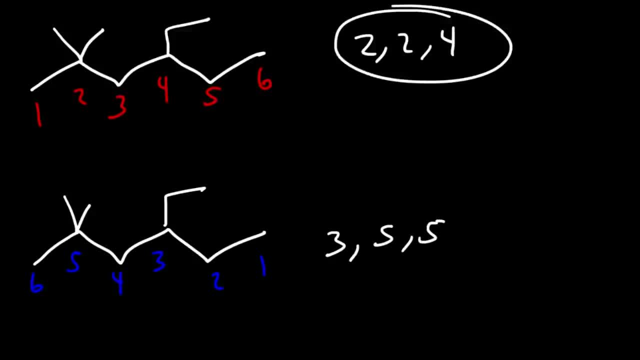 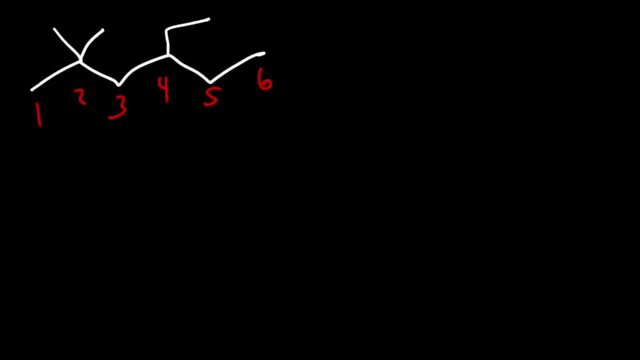 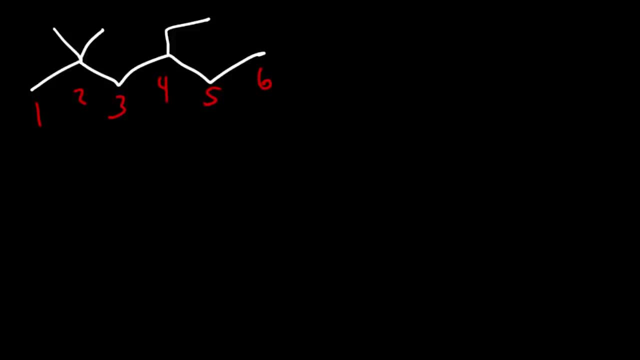 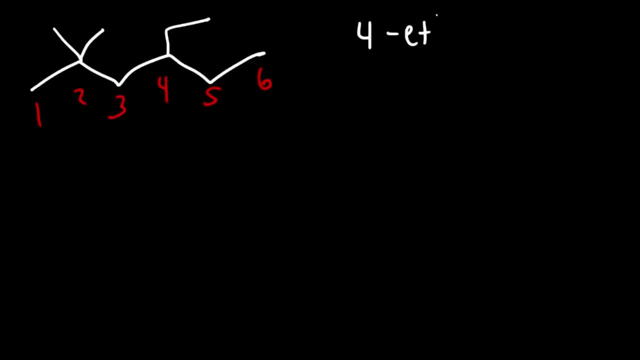 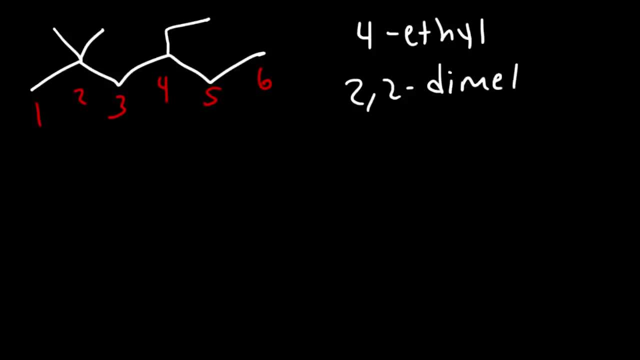 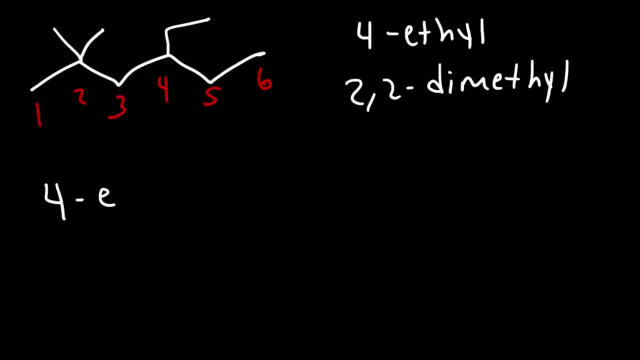 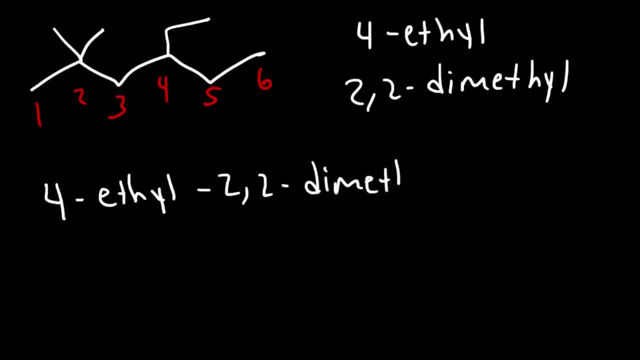 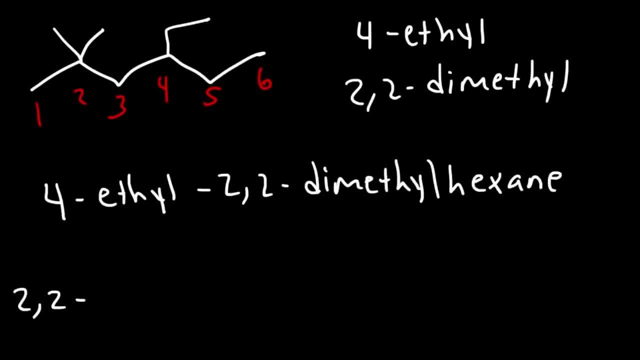 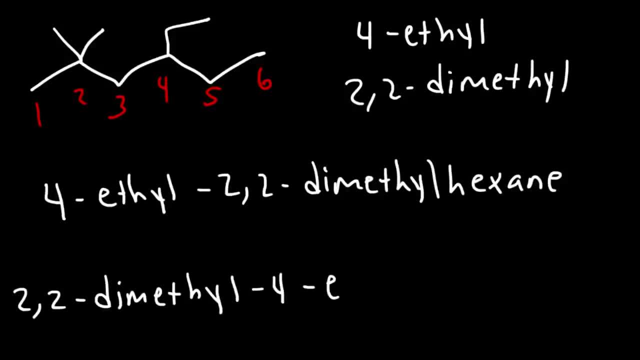 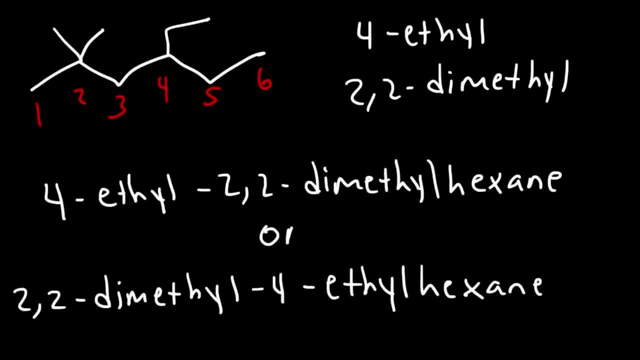 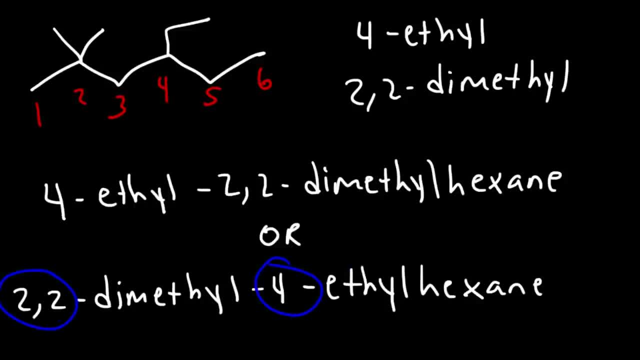 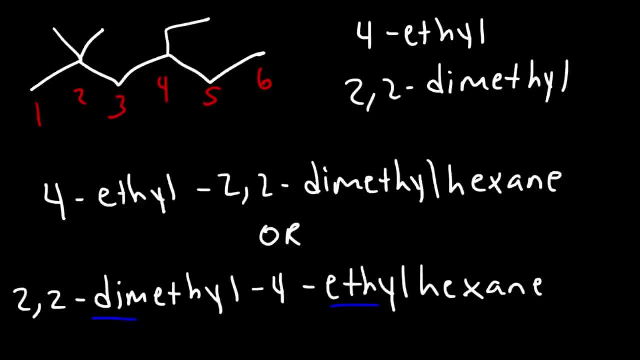